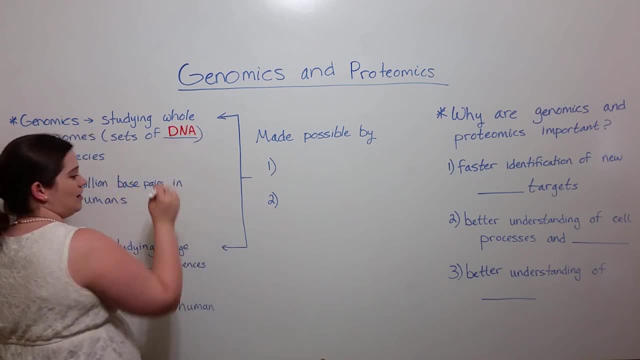 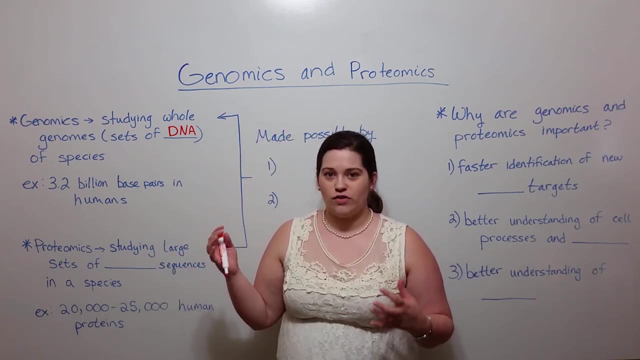 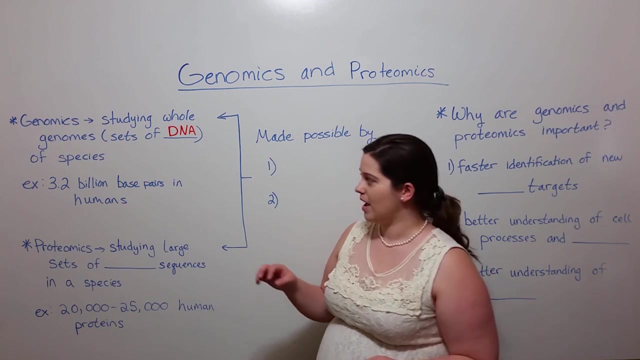 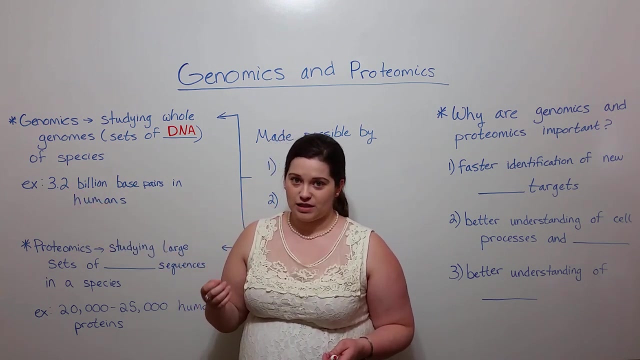 of DNA in a cell. So this tells us about all of the DNA, all of the genetic information stored in a species, And this can be very, very complex. For example, in humans, there are 3.2 million base pairs that make up our genetic information. 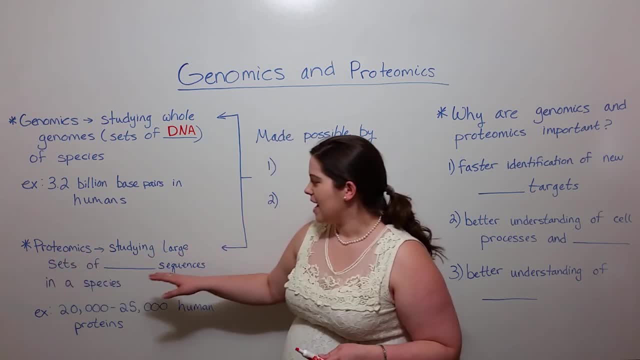 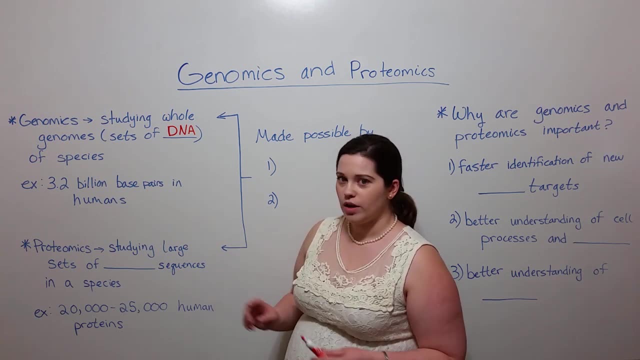 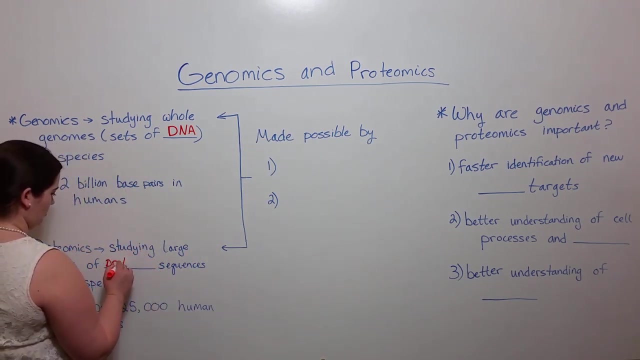 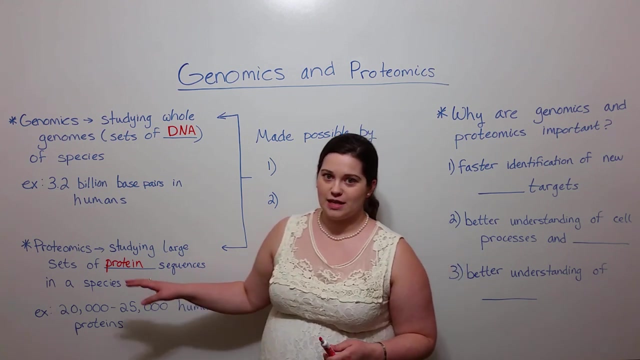 Proteomics is similar. It is also studying a large amount of content. but rather than studying sets of DNA proteomics, studies sets of protein sequences. So this refers to those amino acid sequences that make up the proteins, And the proteins in our cells are the 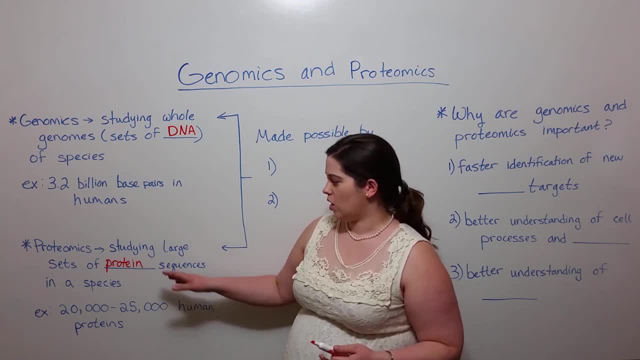 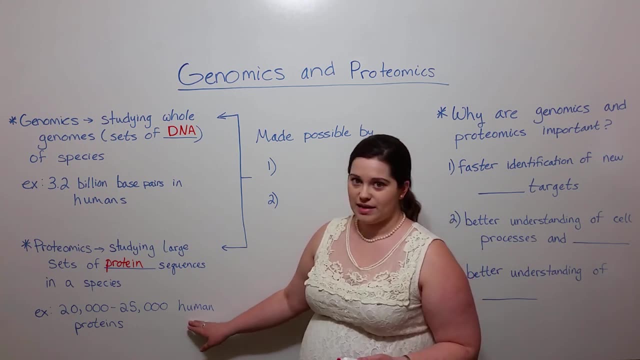 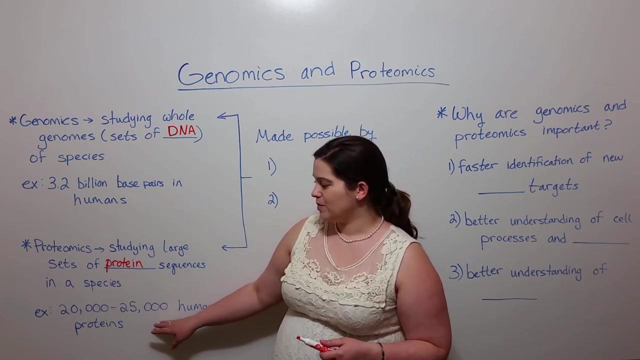 functional aspects of the cells. Proteins are involved in practically every cellular process. For example, in humans there are between 20 and 25,000 proteins And at this point approximately a quarter of these proteins are still unstudied, That is, they've been found. 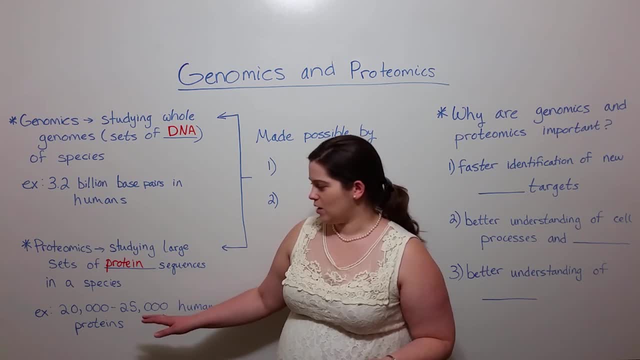 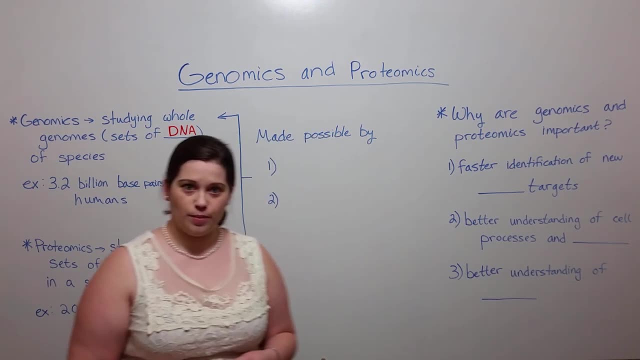 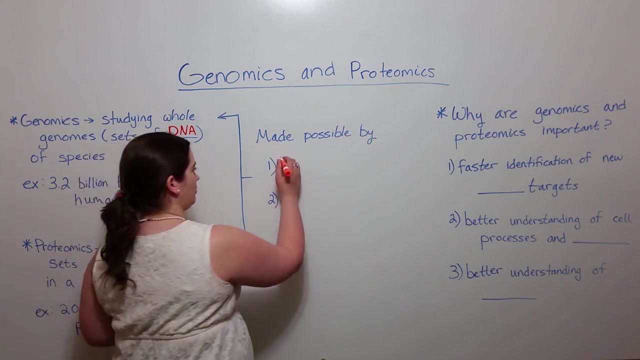 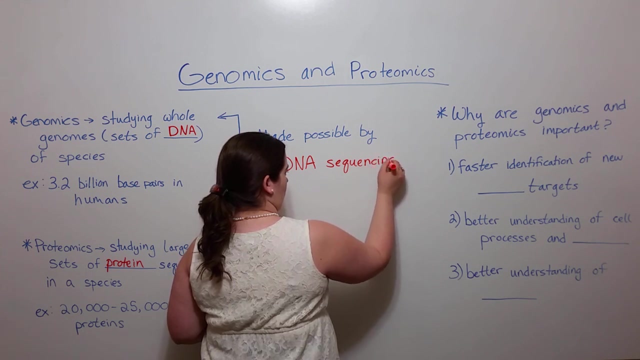 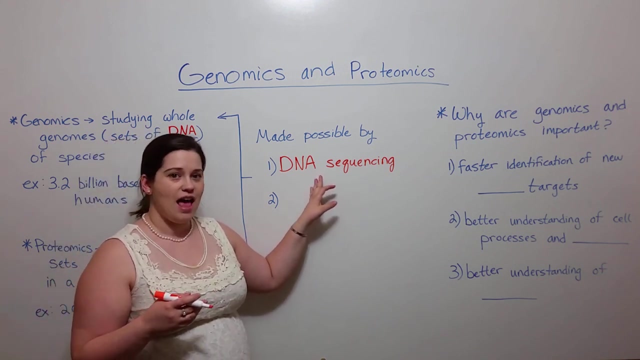 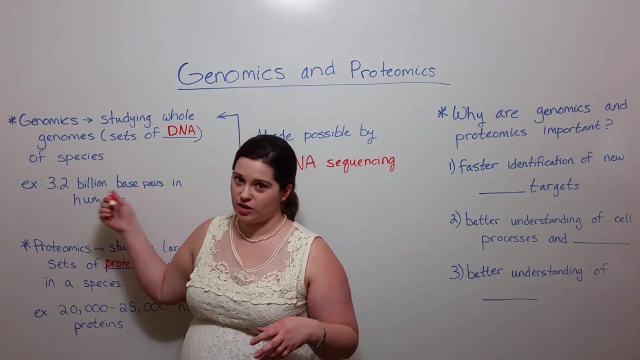 within the cell, but nobody really knows yet what they do Now, genomics and proteomics. what makes these things possible? Mainly two things. Perhaps most importantly is DNA sequencing. DNA sequencing is up-and-coming technology. It's getting better and faster all the time at piecing together not just all of the base pairs in a given genome. 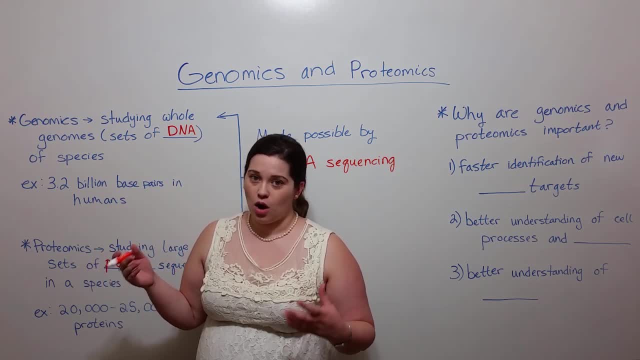 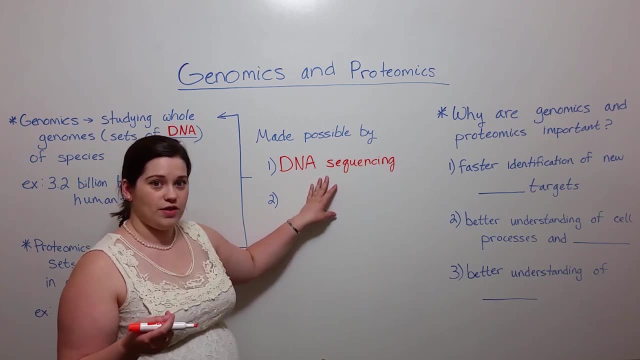 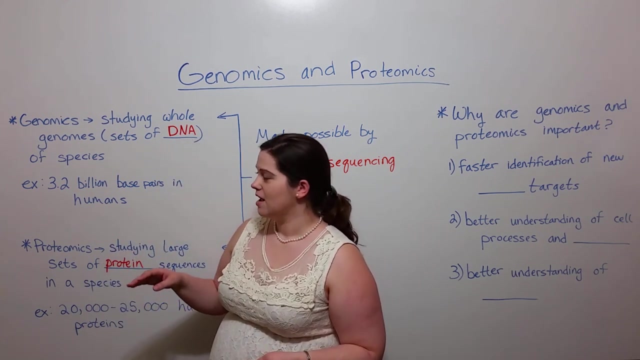 but the order in which those base pairs are put, the order in which they exist. Now, once you know the order of the nucleotides, you can then determine for the protein coding sequences, that is, for the nucleotide sequences that actually code for protein. 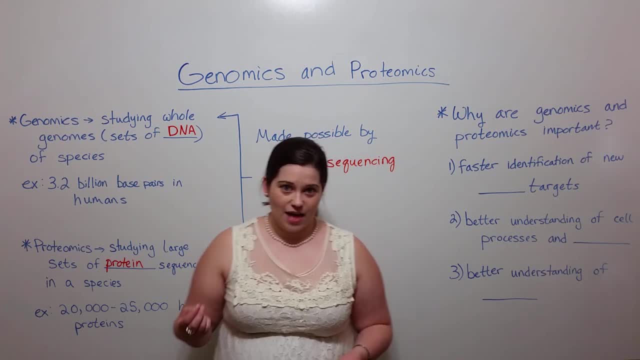 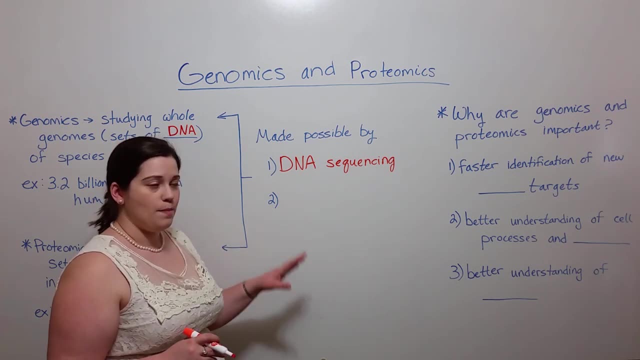 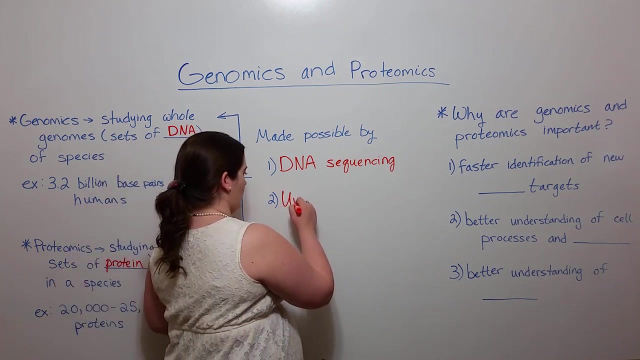 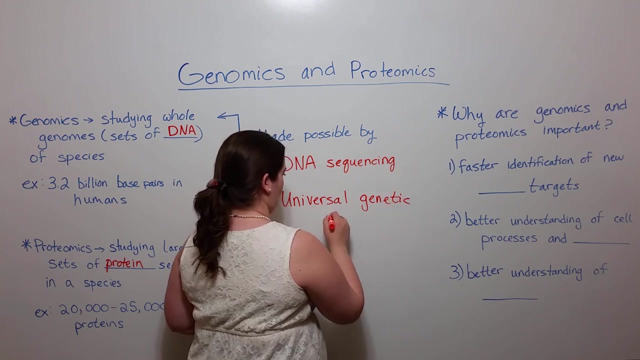 you can determine the amino acid sequence that is coded for by those nucleotide sequences And of course that is made possible by the fact that all organisms share a universal genetic code. If you are interested in learning more about the universal genetic code, 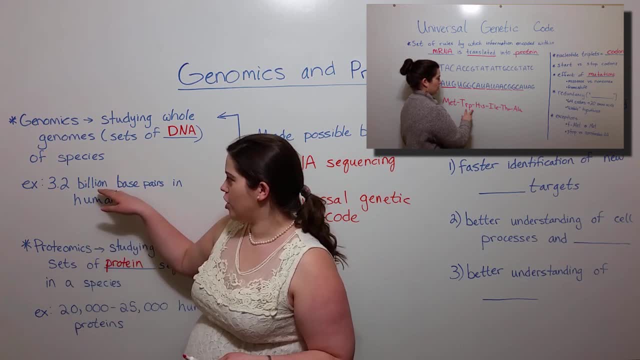 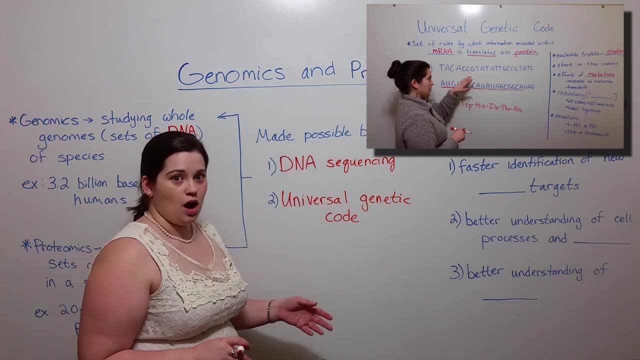 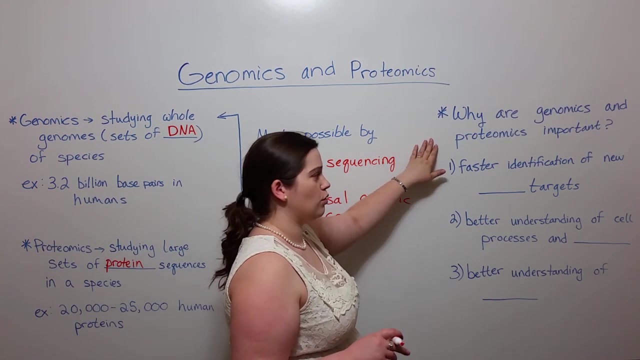 how it works, how it helps us to go from a known base pair sequence or nucleotide sequence to a known amino acid sequence. then see my video on the universal genetic code. But now let's move on to something else. Why are genomics important? 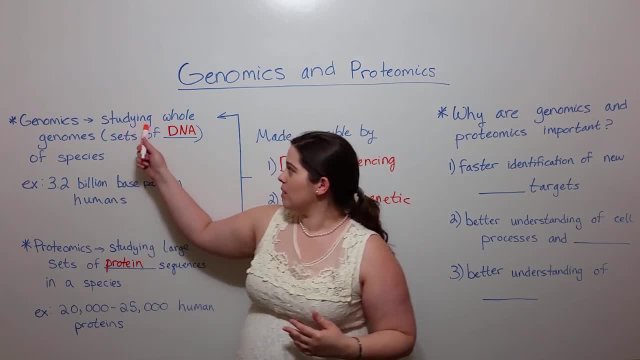 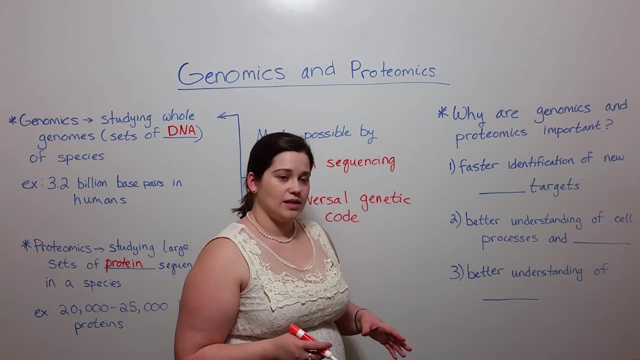 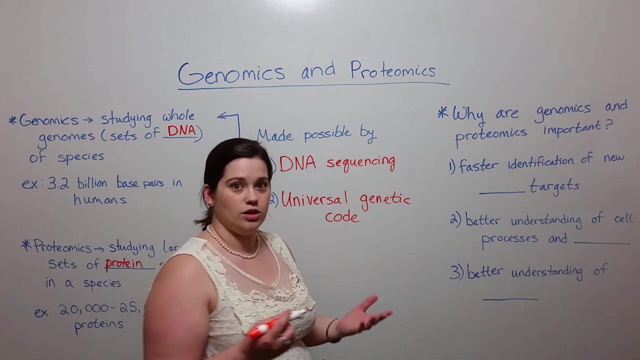 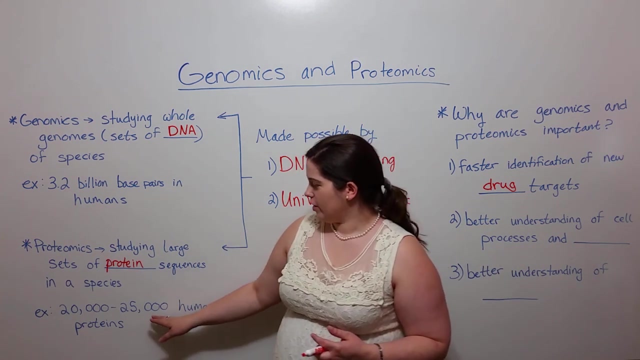 Why are proteomics important? Why do we care about studying whole genomes and studying large sets of protein? Well, a few different reasons. In terms of human medicine, it allows for faster identification of new drug targets. We mentioned earlier the approximately 25,000 proteins. 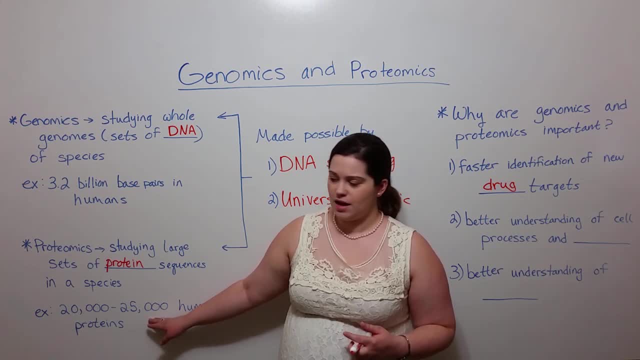 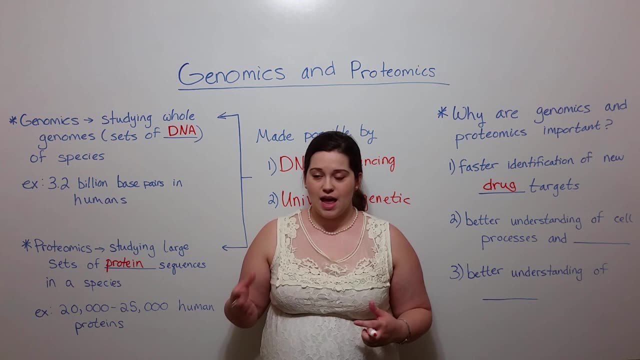 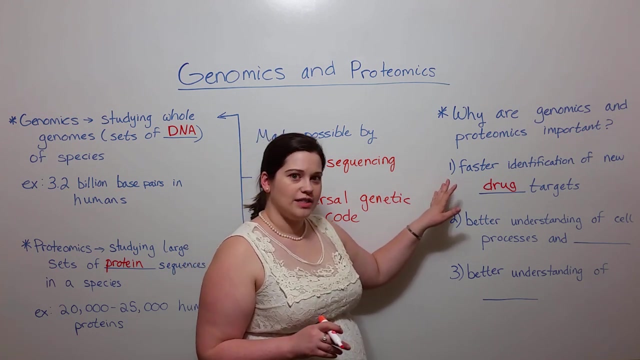 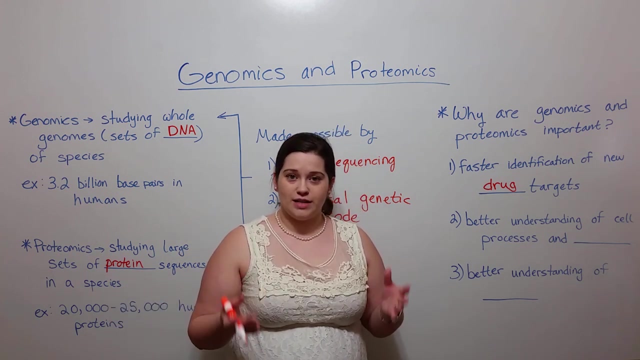 that human cells are capable of. Many of these proteins are essential in various cellular processes, And when something goes wrong with those processes, disease results. And so, by understanding the proteins that are present in our cells and which proteins may need to be upregulated or downregulated, 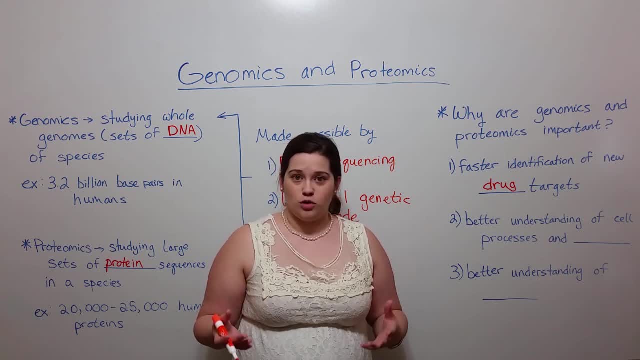 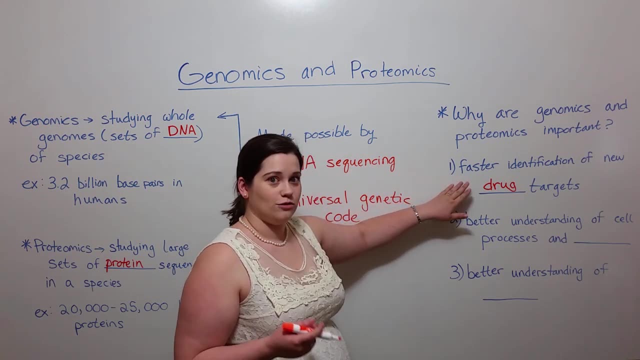 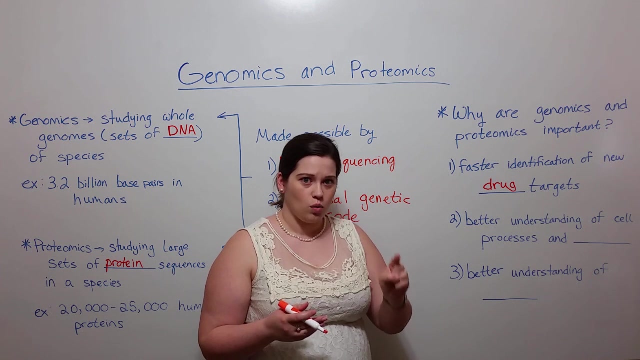 which proteins may need to be prevented from doing certain activities in order to prevent disease. we will have, with the process of genomics and proteomics, faster identification of new drug targets, that is, proteins that we can target with drugs to cure human diseases. 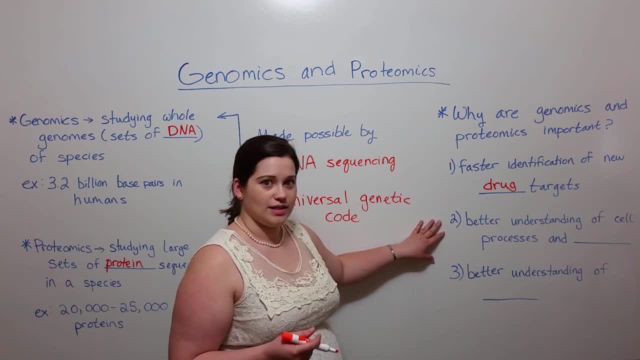 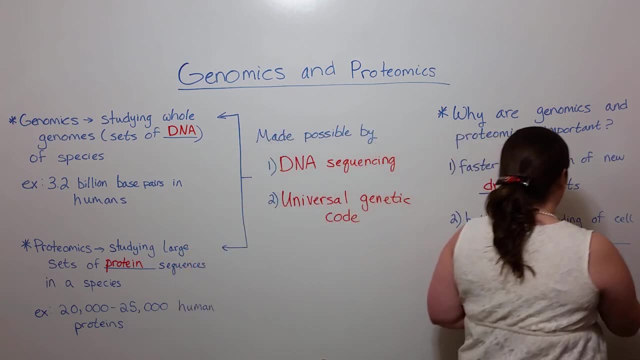 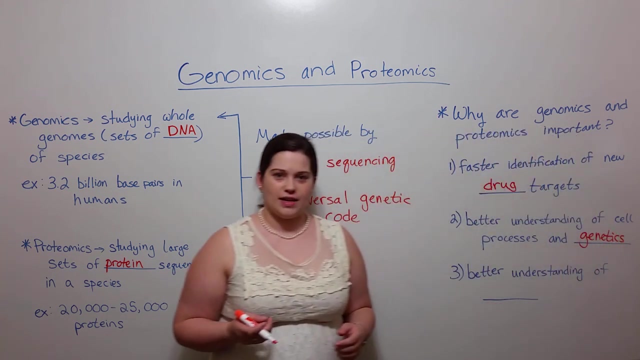 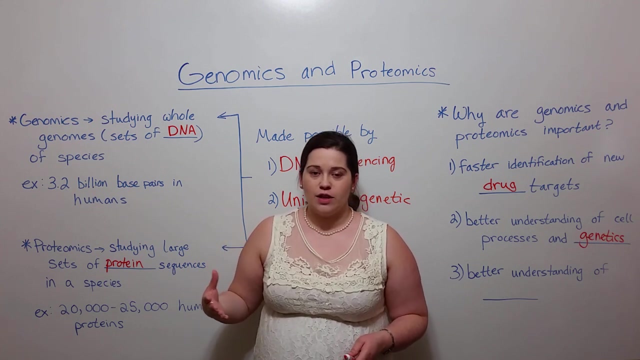 In addition to better understanding of cell processes, genomics and proteomics also give us a better understanding of human genetics. Why do we care? Perhaps the best example of this is that, before the human genome was sequenced, scientists believed that the majority of the genome coded for proteins, And in fact we now.